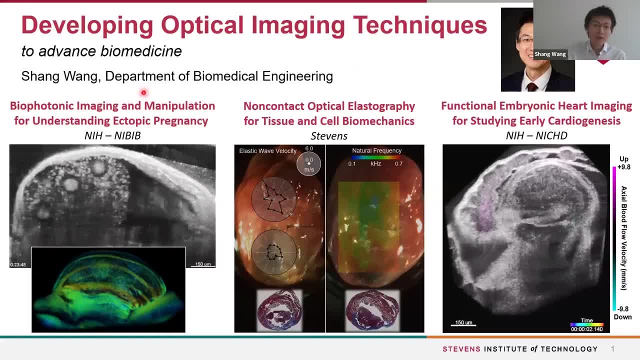 currently have three directions in the lab. In the first direction, we target on the unknown etiology of tubo-ectopic pregnancy, since it's so hard and challenging to study this life-threatening reproductive disorder, especially on how it forms. So our goal is to establish 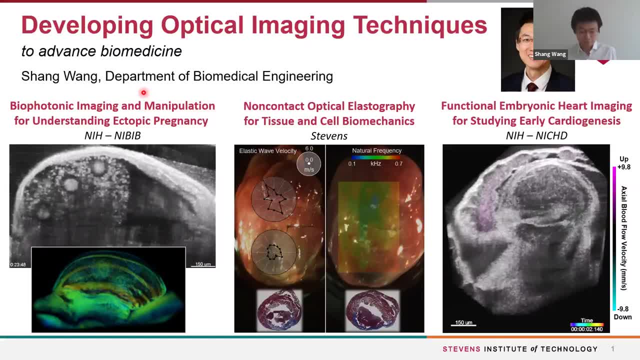 a new intravital in vivo imaging platform that integrates 3D structural, functional and dynamic imaging together with optogenetic control to really address this technical hurdle in the ectopic pregnancy research. So the second direction is on biomechanical imaging, where we develop non-contact optical 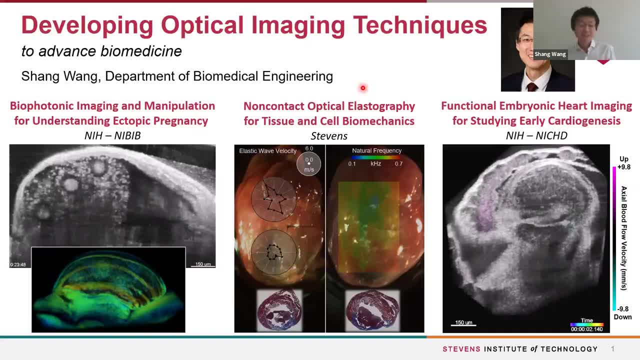 elastography methods. It is well known that the tissue elasticity or stiffness is. a change of those properties is well involved in numerous pathologies such as cancers and cardiovascular diseases. So by imaging and measuring elastic properties of tissue We can enable early detection, better diagnosis. 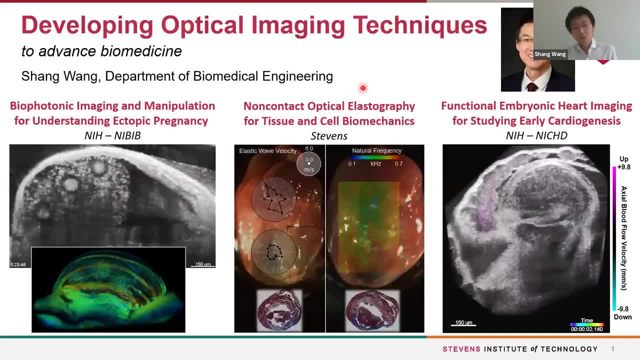 and advanced monitoring of treatment. So, interestingly, stiffness is scale dependent. For example, at an individual cell level, metastatic cancer cells are softer than normal cells, but on the macro level, tumors appear to be stiffer or harder, which can usually be sensed by palpation. So this really indicates the 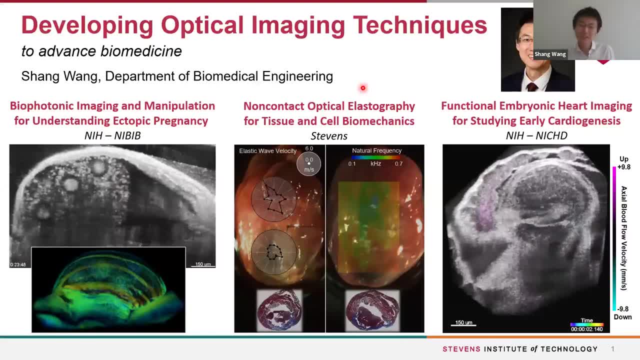 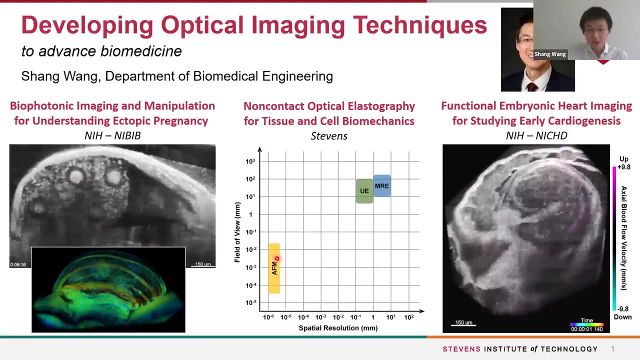 significance or importance of probing and understanding biomechanics at different scales. Currently, existing techniques largely rely on atomic force microscopy that measures subcellular level stiffness, and also ultrasound and magnetic resonance elastography for the organ level analysis. So this leaves really a big gap here. 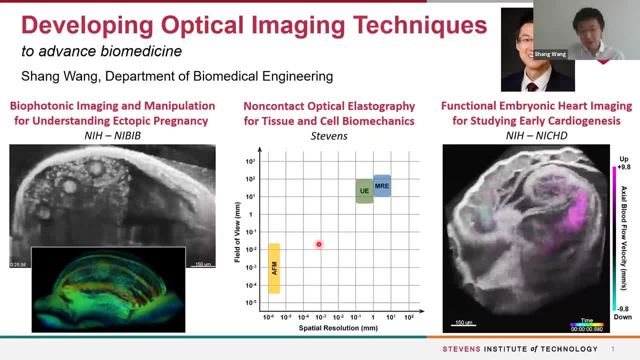 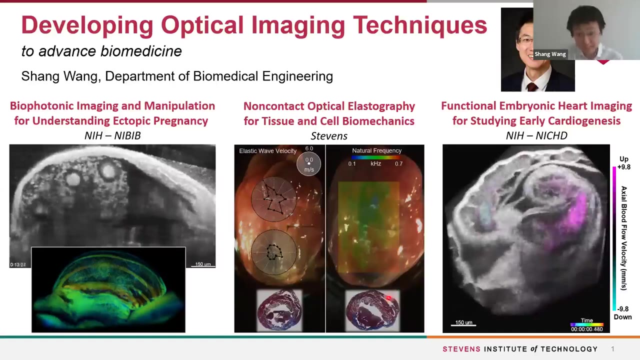 for microscale tissue level assessment. We are using light to develop techniques that can exactly fill in this gap, providing mechanical imaging of cells as a group together under their native environment. So in the example here I'm showing that to understand the biomechanics of myocardial infarction, our method can provide not only 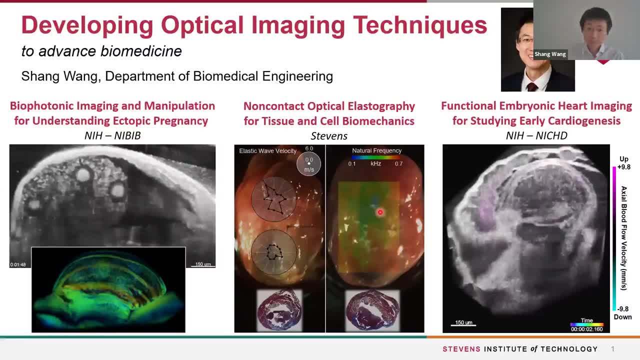 a high resolution mapping of stiffness in the tissue, but also direction, resolved elasticity in the healthy myocardium as well as infarcted region. So we are currently exploring new contrast mechanisms and expanding new applications, and also pushing this technique further for higher resolution and faster imaging speed. 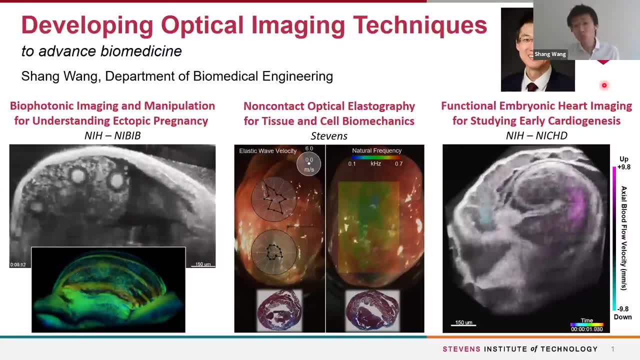 So in the third direction, we are collaborating with Irina's lab at Baylor College of Medicine to study the biomechanics of myocardial infarction. So the biomechanics of myocardial infarction is used on unbiased cells and in this particular case we are using the biomechanics of early mammalian cardiogenesis. 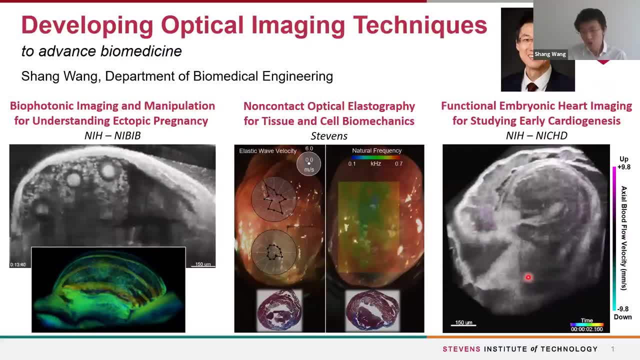 for better understanding of congenital heart defects, which is the most common birth defects. So specifically, my lab works on quantitative imaging of the hemodynamics shown here in the beating heart And most recently we have established a new approach for the pumping analysis in this tubular heart. 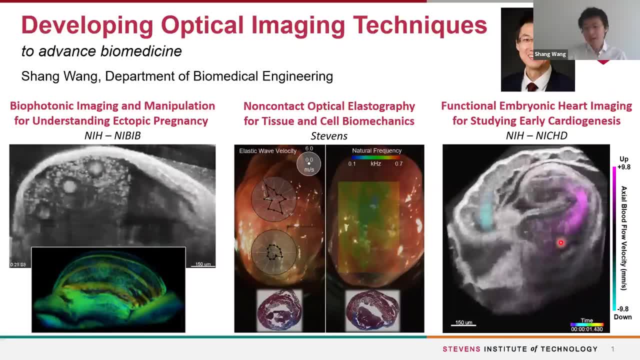 particular flow patterns are generated. So currently we are developing methods for spatial temporal analysis of the flow induced shear stress on the endocardium to better understand how this, basically better understand this mechanical factor in the mechanotransduction involved in early heart development. So I think in the next four minutes or so I'm going to into a 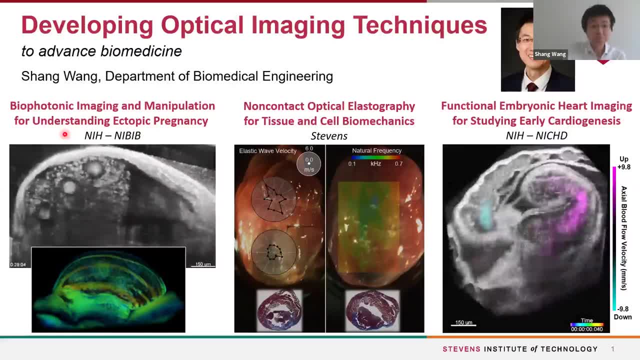 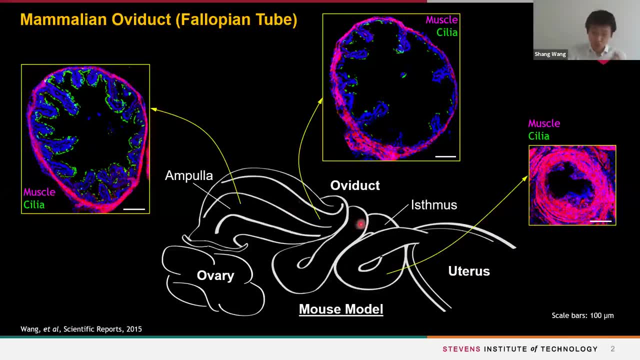 little more details in the first direction. The mammalian oviduct, or can also be called as fallopian tube, is a tubular structure that connects the ovary and uterus. There are primarily three reproductive events taking place in the oviduct: The transport of sperm and oocytes, fertilization and embryo. 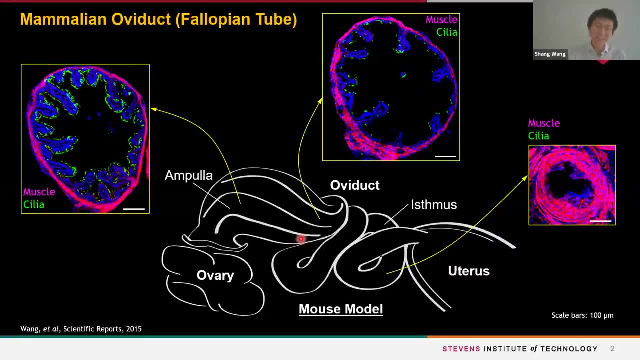 transfer. So, as you figure out, there are a lot of transporting activities involved, so there need to be motors. There are two sources of force in the oviduct. One is the contraction of smooth muscles located on the wall. The other one is a bit of motile cilia and 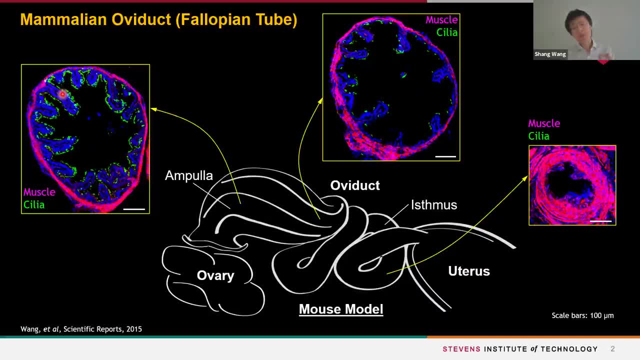 the acafilia of the lumen. So, despite a long history of research, how these two motors or sources of force contribute or regulate the reproductive process inside a mammalian oviduct is very difficult to say without any is still not clear. 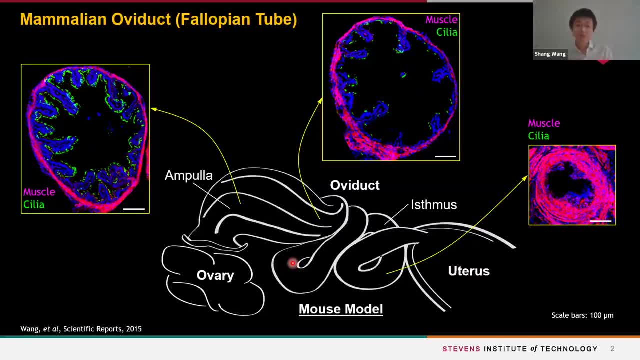 A primary reason is that most studies were based on in vitro or ex vivo tumor settings, just like these histologies. As a result, today very little is known about how a normal reproductive process looks like inside the mammalian oviduct And in terms of disordered conditions. 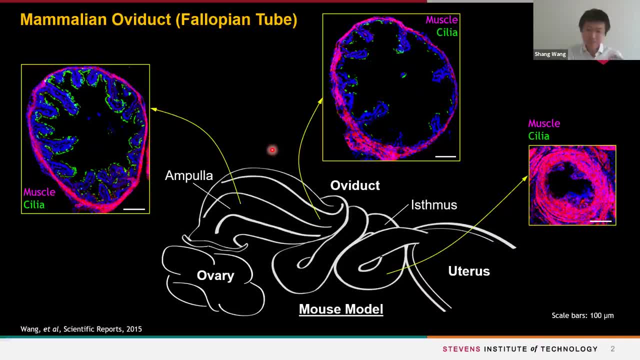 such as ectopic pregnancy. it has been nearly impossible to investigate the dynamic and functional parts of this reproductive process that has been disrupted in the mammalian oviduct. So this is exactly the missing component of current reproductive research And unfortunately there has been no imaging tool. 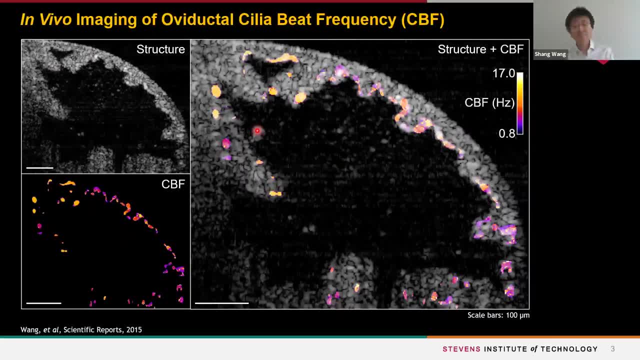 allowing us to do that. So over the years we have been continuously working to resolve this technical challenge and to make it possible to for in vivo studies of mammalian oviductal structure, function and dynamics with a high resolution. 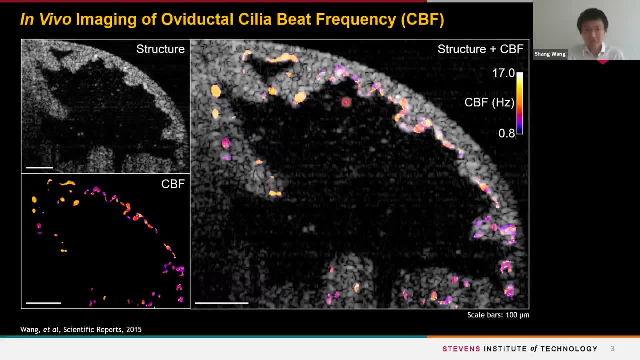 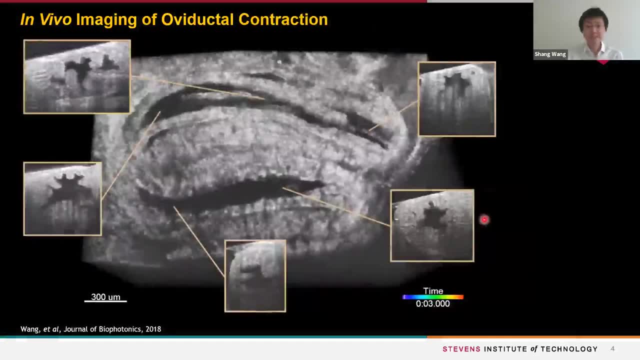 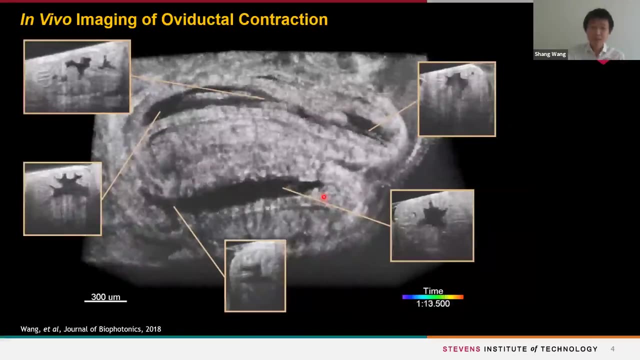 And this includes, as shown here, microscale mapping of the CW frequency on the luminal epithelium and in vivo 3D assessment of the oviductal smooth muscle contraction and also the contraction wave propagation, As well as 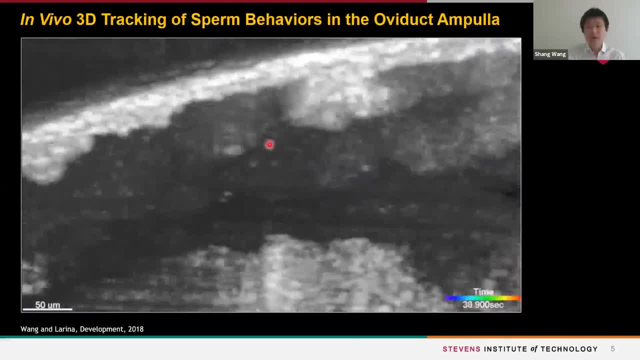 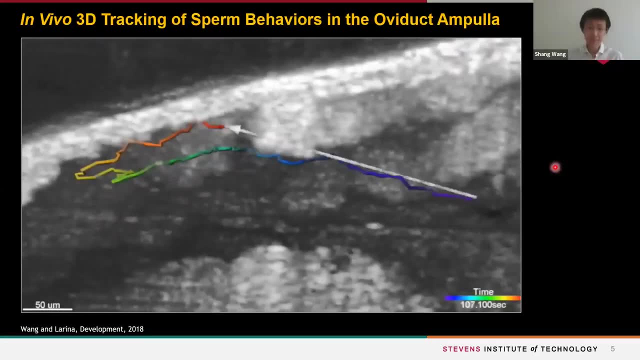 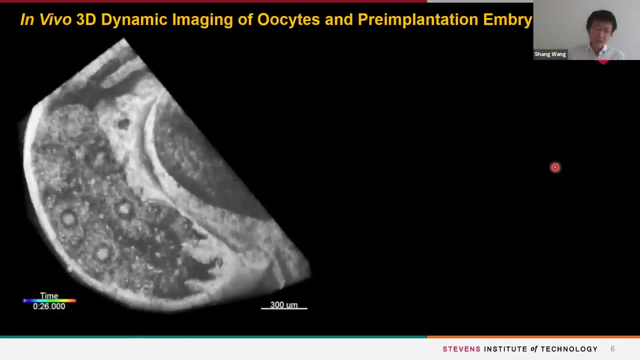 in vivo 3D tracking of sperm inside the oviduct ampulla, showing a number of never-before-seen sperm behaviors in the native foliation environment. So most recently we have achieved this first in vivo 3D imaging of the dynamics of oocytes and preimplantation embryos. 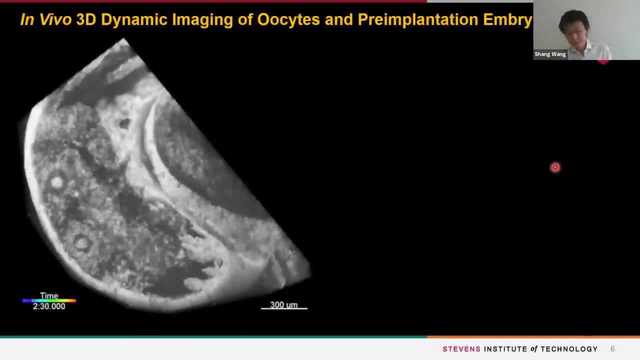 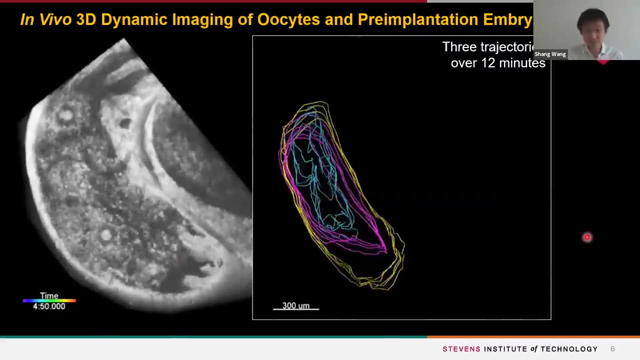 as they are transported through the oviduct And in the example shown here, it shows that the cumulus oocyte complex has an unexpected circular movement inside the oviduct ampulla And their trajectories are spatially distinct. So this imaging 3D imaging approach. 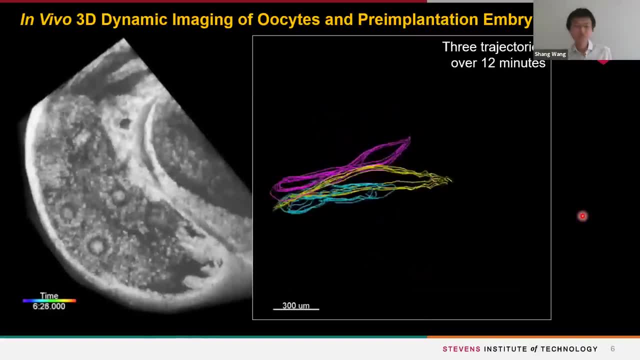 really opens the door for in vivo studies of embryo retentions in the oviduct as a prerequisite. So this imaging 3D imaging approach really opens the door for in vivo studies of embryo retentions in the oviduct as a prerequisite for the oviduct. 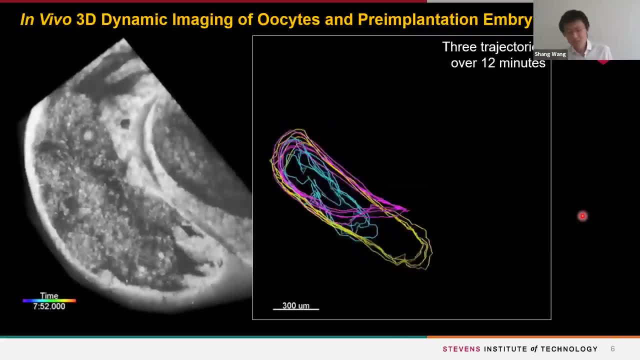 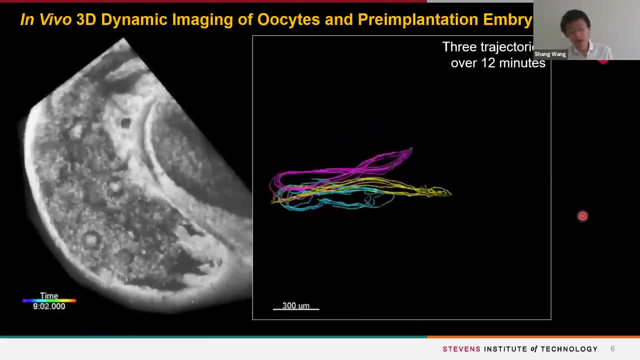 So this imaging 3D imaging approach really opens the door for in vivo studies of embryo retentions in the oviduct as a prerequisite for the oviduct, And we're currently developing manipulation and interventional approaches that can be combined together with our imaging techniques. 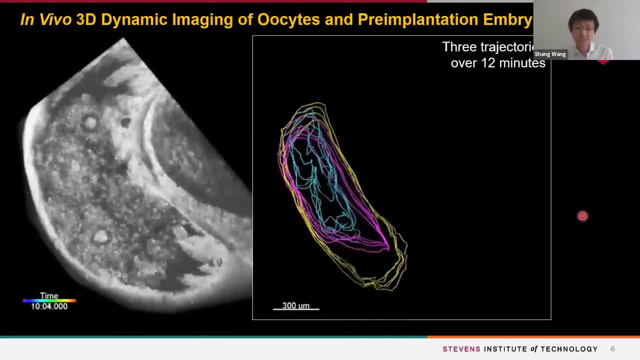 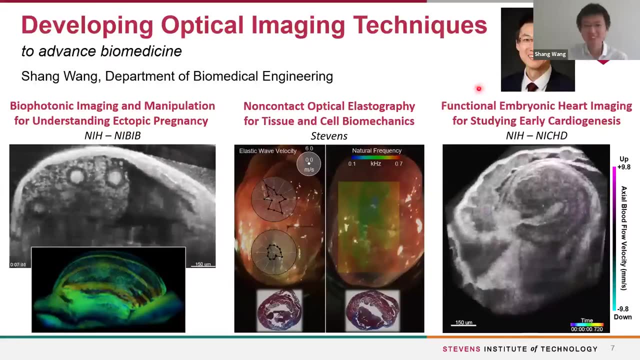 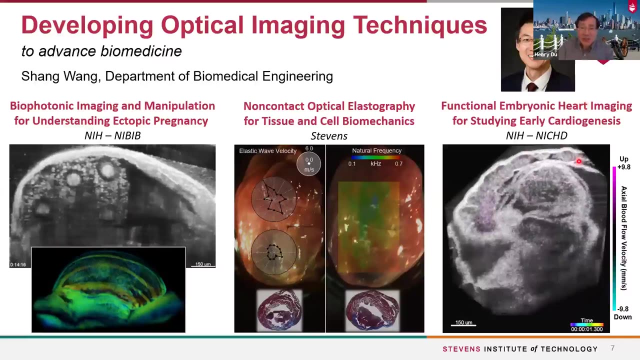 to elucidate the functional cause of embryo retention in the mammalian oviduct. So that's all And thanks for listening. Happy to answer any questions. Well, thanks much, Sean. Very exciting work. I don't see any questions submitted. 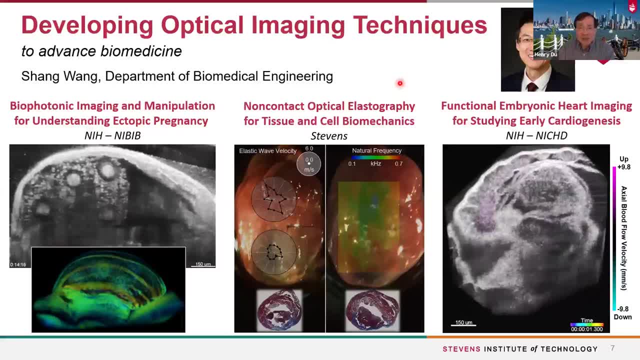 Let me try and ask a very naive question anyway. So, when it comes to optical imaging, right, Because of limited tissue penetration depth, unless you do endoscopy-based imaging, you can hardly produce the images that you are showing. So is that the technique that you use? 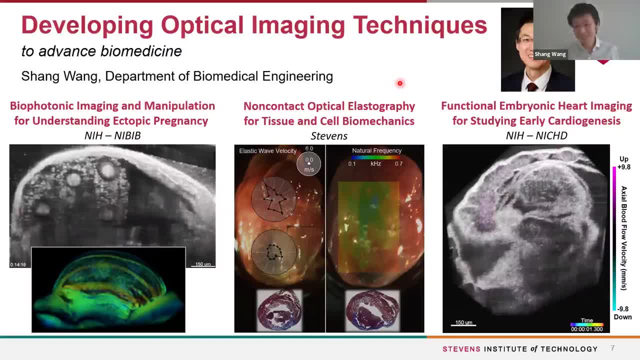 Well, yes, it's very right. So for optics, getting into deep inside the tissue is pretty hard. So first of all, we are working with the mouse model, So to get the knowledge out, basically with all the tools that already exist with mouse model. 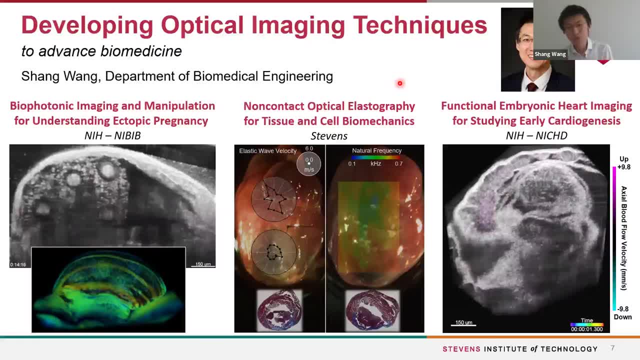 and also still to really approach to the reproductive organs in the mouse. it's still very, very hard. So what we did is we employed an intravital window that sort of can provide us the, basically the light, provide us opportunity to deliver the light into. 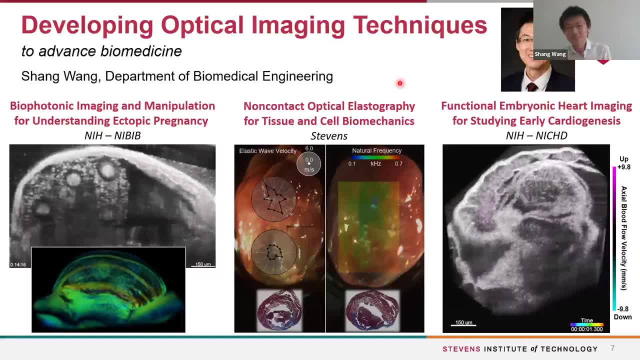 and get the image out. So that's basically the way we go inside the body And, as you said, there's endoscopic approaches that combine with optical imaging that can really give you know images inside the body. 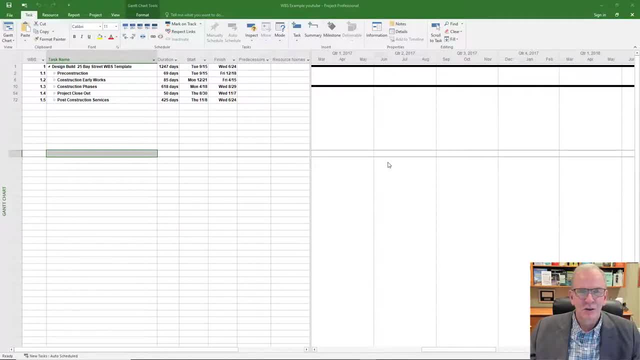 Hi, I'm Tom Stevenson and welcome to Microsoft Project Made Easy. Today we're going to be looking at work breakdown structures, particularly within a construction business, and how you can set them up, how they work, how you should think about them in MS Project. 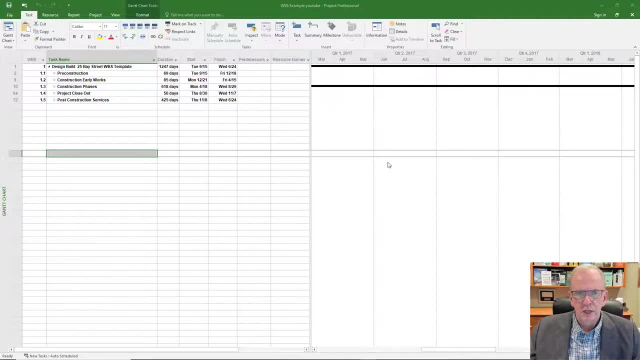 I've done other videos on my YouTube channel just on work breakdown structures in general from a project management perspective. In this video I'm really sort of applying that to Microsoft Project. So on your screen you can see I've created a little bit of a work breakdown structure here. It's actually fairly in-depth if we open it up, but this is kind of like at a high level. 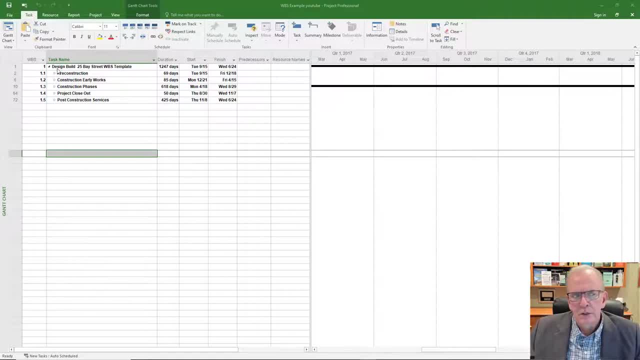 And really what you've got to get used to is that you've got what Microsoft Project refers to as summary tasks, which are headings, And so underneath a heading like this would be your overall project. So say I had this multi-story building on 25 Bay Street, this would be like the top level heading that you would have. 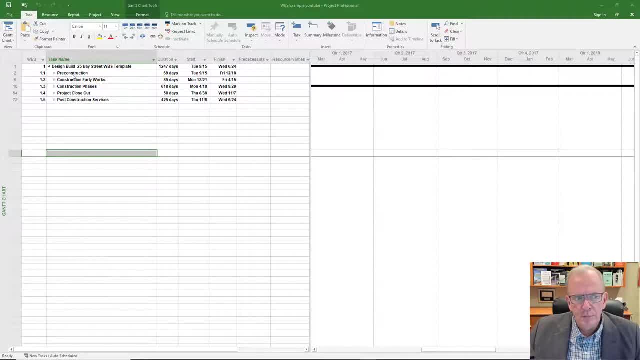 And then underneath it, you would have the following: Well, you can do whatever you want with it, like in a construction project, but very often you'll probably find headings that require a lot of work, So you could have a lot of work. 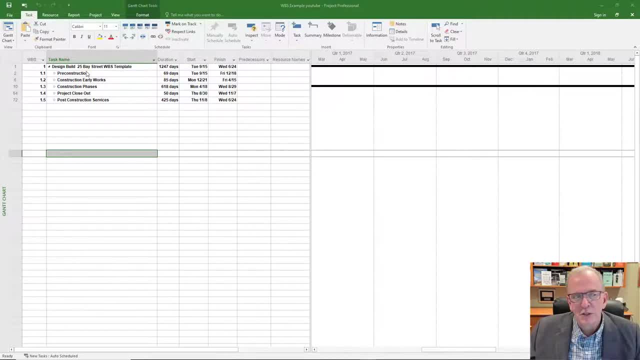 So working on a site will involve something like this: Everything that's going to be before construction, so pre-construction, early works, so these are things like preparing the site, that you're actually doing some things on, but not direct the construction process. 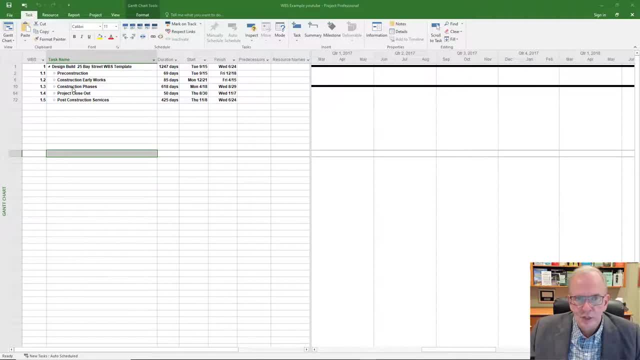 And then the construction phases or construction process. You can name it what you will that way. But as long as it's incorporated, what you try to do is you try to standardize it within your business. So you can name it what you will that way.